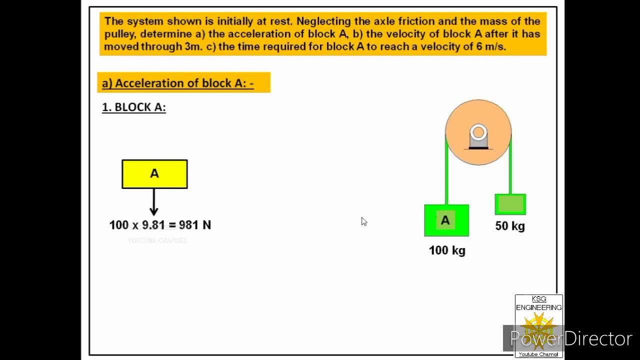 downward direction, then the next force which we have to represent in the free body of block A will be tension in this cable. so that will act in upward direction. so let us consider that as T. so in the free body of block A there will be only two forces. one is the weight of the block acting in downward direction. 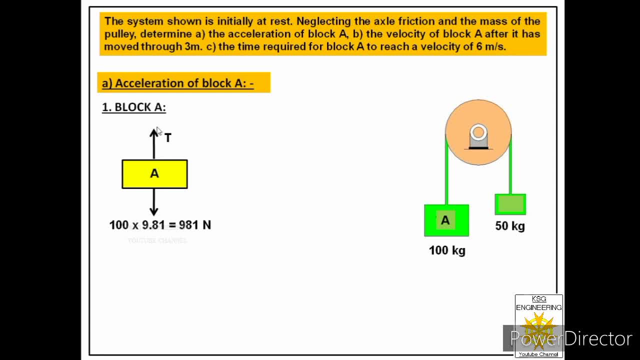 second is tension in the string acting in upward direction. now we know that in this situation, tendency of block A is to move in downward direction. so motion of the block A will be in downward direction. so we can say: this system is equivalent to the motion of block A in downward direction. now we can say that this 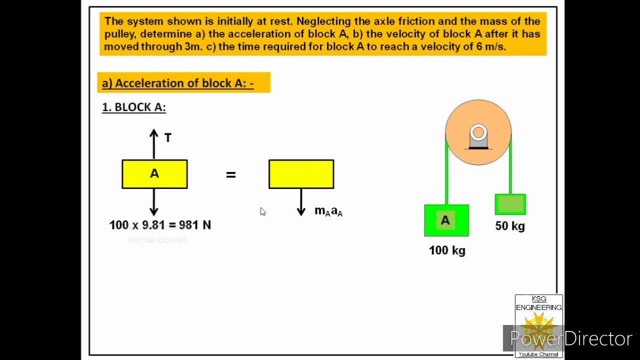 system of forces, that is summation F is equal to ma and there are no forces acting in the free body in x direction. so only one equation is applicable for this block, that is submission f: y is equal to ma. We will consider those forces positive which are acting towards the motion of the block and will consider other force. 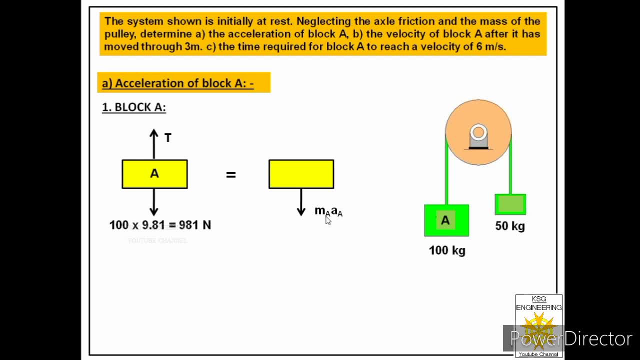 negative, which are acting against that motion. so let us apply the equation that is summation: Fy is equal to ma, so we have two forces. weight is acting towards the motion. so let us take this as positive. tension is acting opposite to motion. let us consider this as negative. it means equation will be: 981 minus t is equal to ma aa. 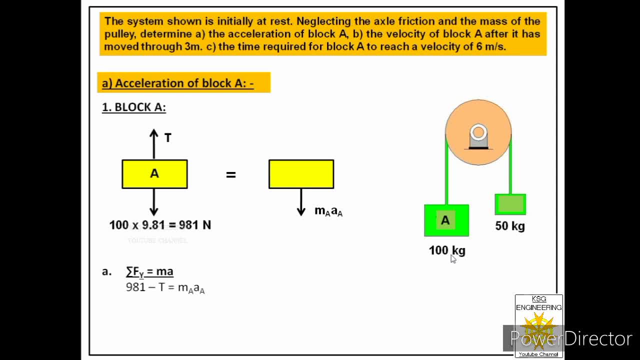 we know the mass of block a as well, which is 100 kilogram. so this equation will further reduce to 981. minus t is equal to 100 aa. so in this equation we have two unknowns. one is tension in the cable. second is acceleration of block a. so let us call this equation as equation number one. 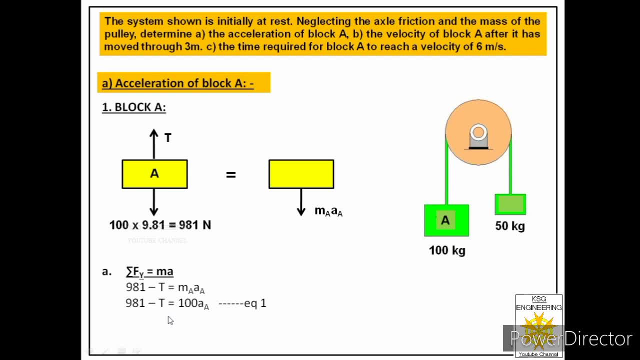 so as we have two unknowns in this equation, so we cannot solve this equation now. we have to take the help of the free body of other block. so let us draw the free body of block b, which is of 50 kilogram, and in the free body of block b we have to first represent its weight. 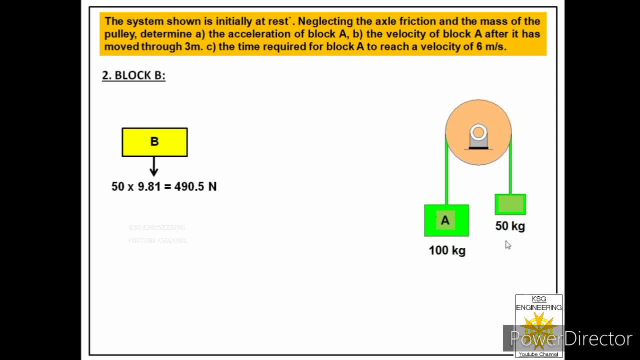 which will act in downward direction. its mass is given to us as 50 kilogram. it means, in order to convert that into weight, we have to take the weight of the free body of block b and we have to multiply 50 by 9.81, so its weight will be 490.5 newtons. and in the free body of block b we have to. 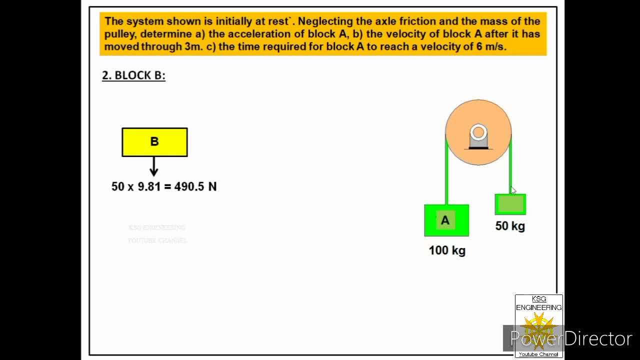 show another force which will be tension in this cable, which will act in upper direction. so we have to show that tension. also let us label that as t, which is same as that of the tension we have shown in the free body of block a, because we are using same cable over here. 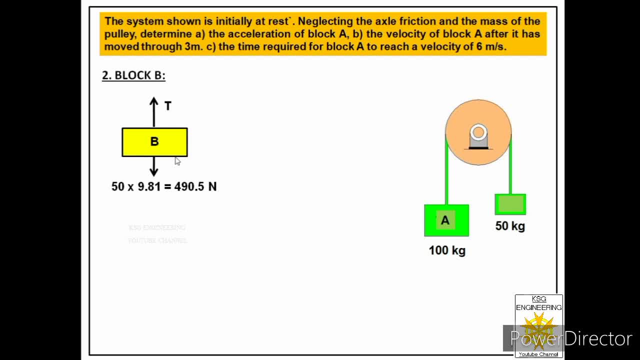 so we have to write t in our function in the free body of block b. let's write t in our function now. in the free body of block b there are only two forces. one is its weight acting in downward direction. second is tension acting in upper direction. now we know if this block is moving. 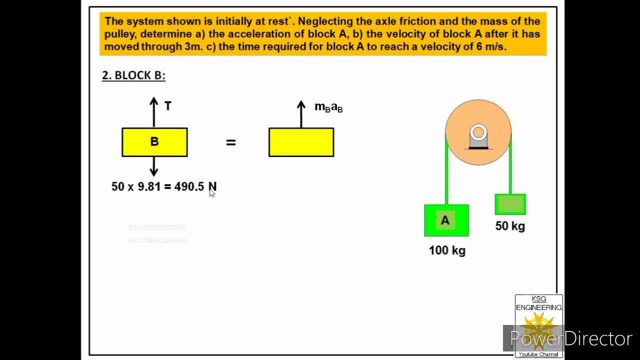 in downward direction, then block b will move in upper direction. that means this system will be equivalent to the acceleration of block b in our direction acting on block B. so only one equation will be applicable, that will be: summation FY is equal to MA, so let us apply that equation. summation FY is 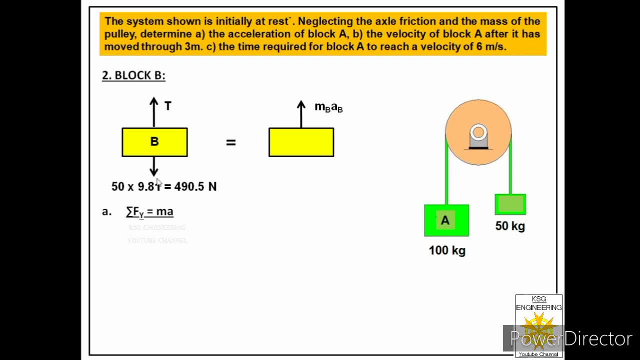 equal to MA. so over here two forces are acting in Y direction, so we will consider that force as positive, which is acting in the direction of motion. so it means equation will be equal to T minus 490.5 is equal to MB AB. now we know. 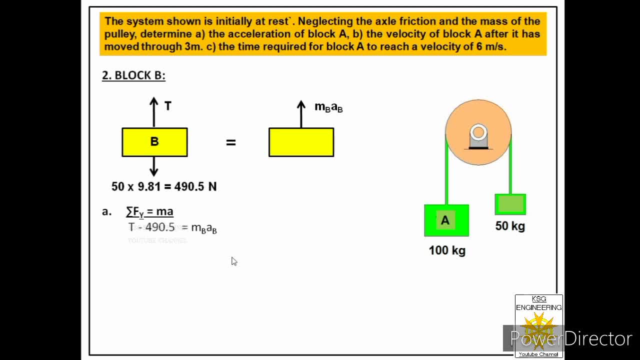 the value of the mass of block B, which is 50 kilogram. so this equation will reduce to: T minus 490.5 is equal to 50 AB. so this equation further will reduce to: T is equal to 490.5 plus 50 AB. so in this equation we have two. 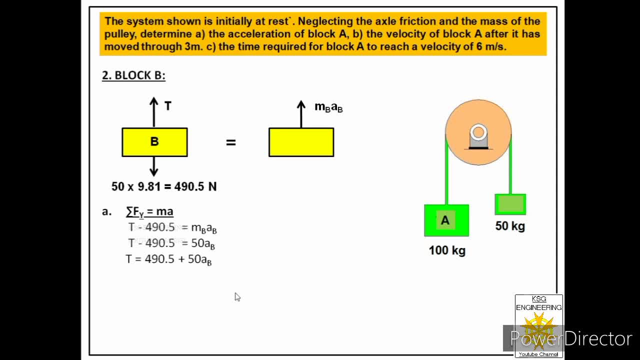 unknowns- T and AAB. but in the free body of block A we have got one equation which is in terms of T and acceleration of block a. Now in this equation we have found the value of tension, that is t. So we will put this value in that equation, that is equation number 1.. So when we will put this value in? 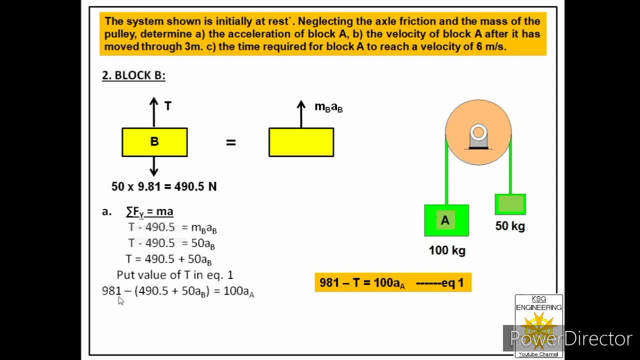 equation number 1. we will get another equation, as 981 minus 490.5 plus 50ab is equal to 100aa. Now in this equation still we have two unknowns: One is ab and second is aa, So we cannot solve. 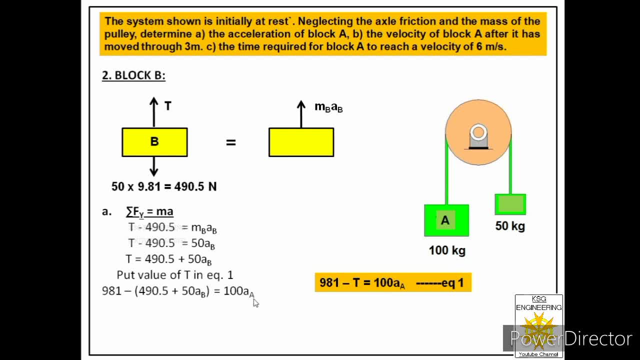 this equation. It means we have to find relation between acceleration of block a and acceleration of block b, And we know in this system both the blocks are connected to a single cable. That means magnitude of the acceleration of block a will be equal to the magnitude of 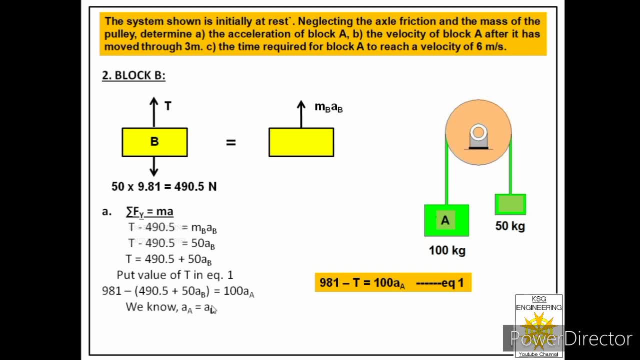 acceleration of block b. So we can say the magnitude of acceleration of block a is equivalent to the magnitude of acceleration of block b. So in this above equation we will replace acceleration of block b by acceleration of block a. So this equation will reduce to 981 minus 490.5 plus 50aa is equal to 100aa. 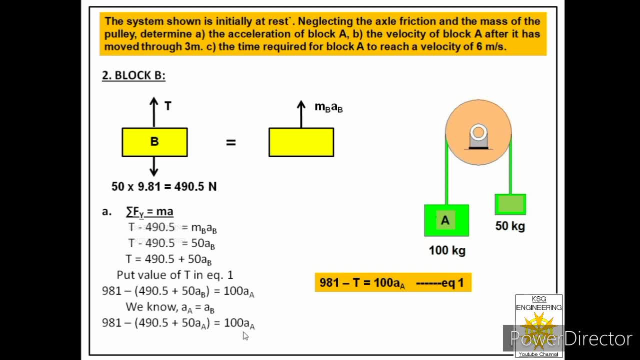 Now in this equation we have only one unknown, that is, acceleration of block a. So we can solve this equation and we will get the value of acceleration of block A as 3.27 m per second square. Now, after this, we have to find B part. 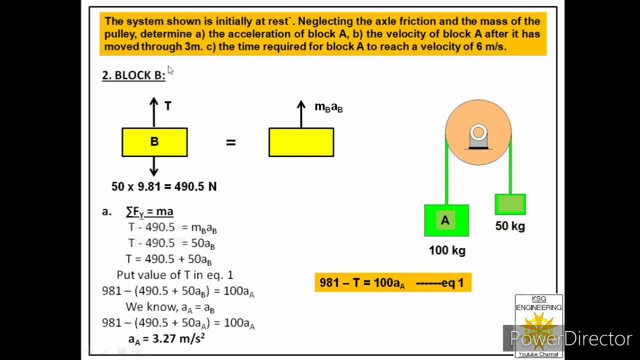 In the B part we have to find the velocity of block A after it has moved 3 m. So we have to find velocity of block A after it has moved through 3 m. Now we know block A is moving in downward direction. 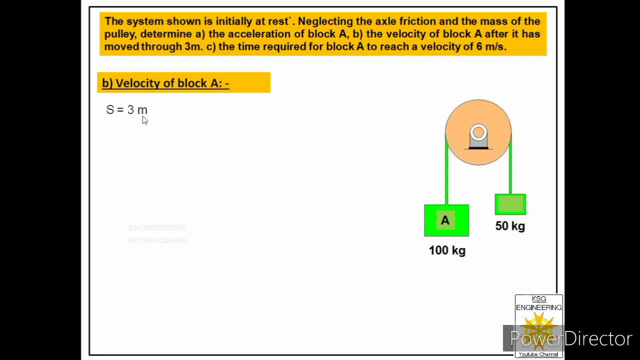 So distance is given to us as 3 m And the initial velocity of the block is 0, because it is mentioned in the quotient that system shown is initially at rest, And acceleration of block A we have already found as 3.27 m per second square. 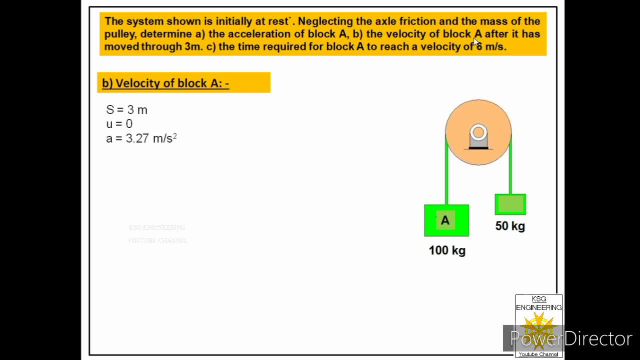 And we have to find the final velocity of block. A means after the travel of 3 m. It means we will apply equation V square minus U square is equal to 3.. So this equation will further reduce to: V is equal to 2, A s under root because U is 0 over here.